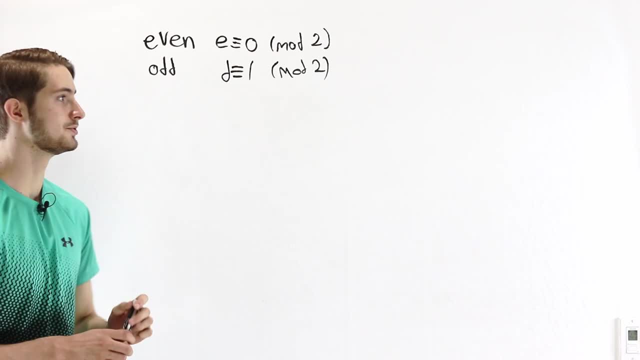 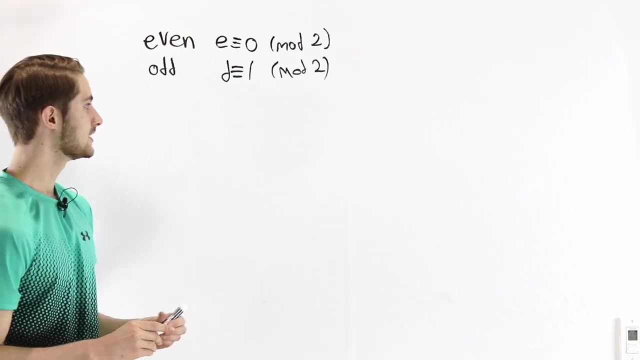 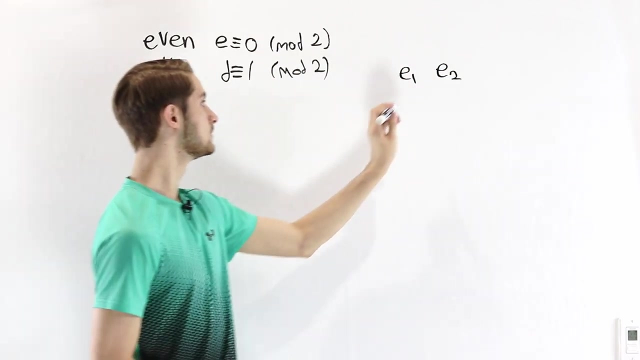 First let's take a look at some properties of sums. We know that we can add the two numbers on the left and right sides of modular congruences. So let's think about if we have two even numbers, E one and E two. what is their sum? Well, we know E one plus E two. both of those are congruent to. 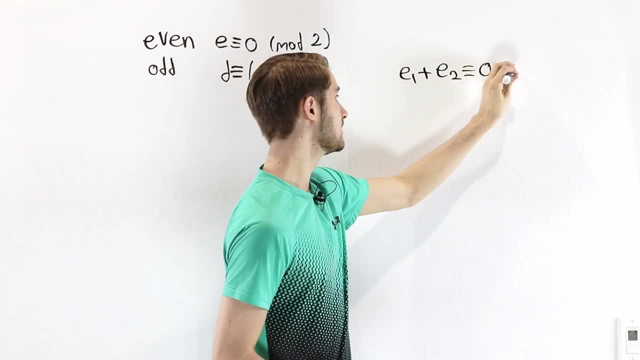 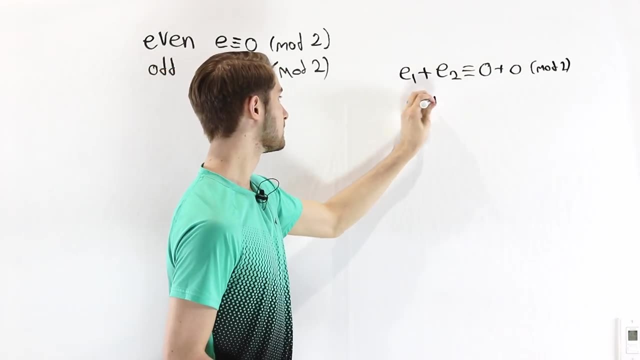 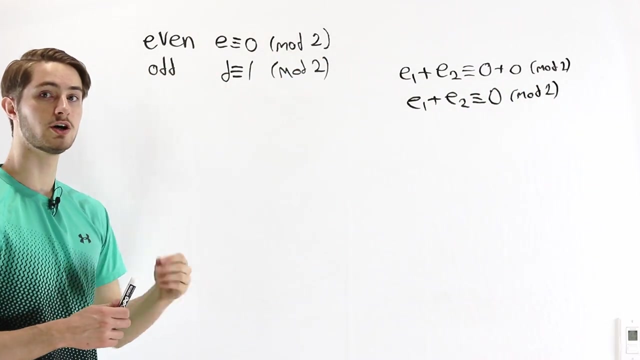 zero. So their sum is congruent to zero plus zero mod two. And we know that zero plus zero is of course zero. So E one plus E two is congruent to zero mod two. Now we know that if any number is congruent to zero mod two, then it is even, And therefore we've shown that the sum of two even. 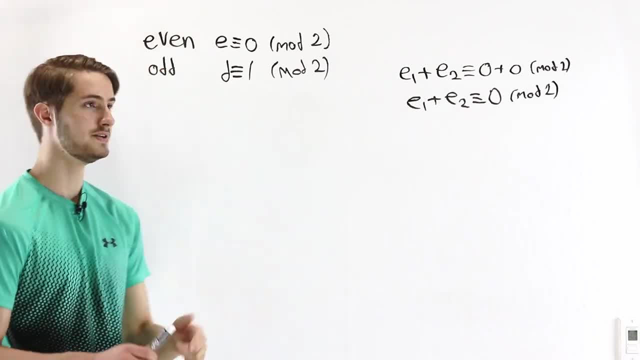 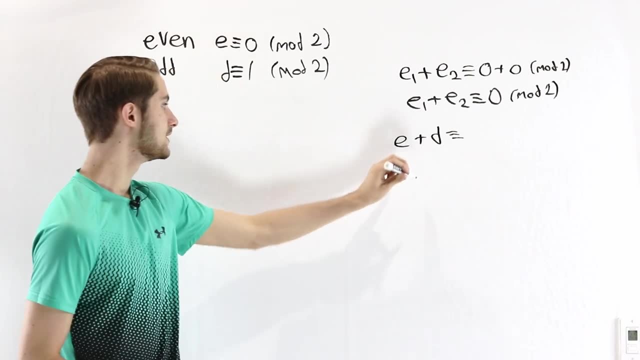 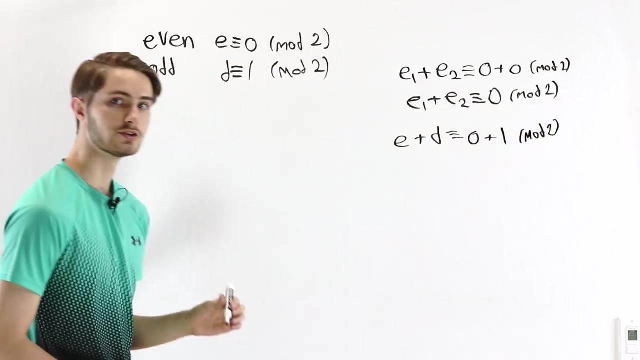 numbers is always an even number. Next, let's look at an even plus an odd number. So say we have even plus an odd number. We know that an even number is congruent to zero and an odd number is congruent to one mod two. So from here on the right side, we have zero plus one, So an even. 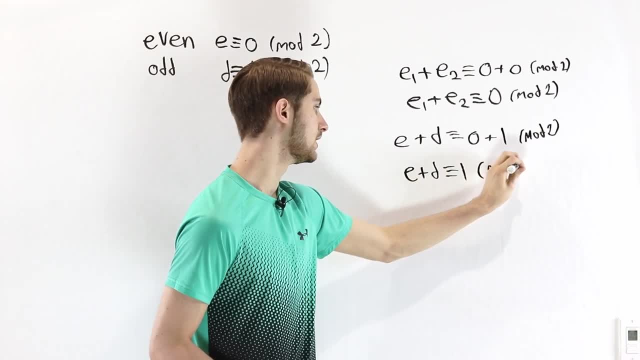 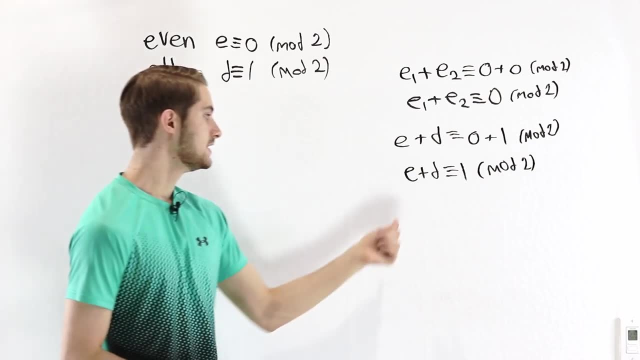 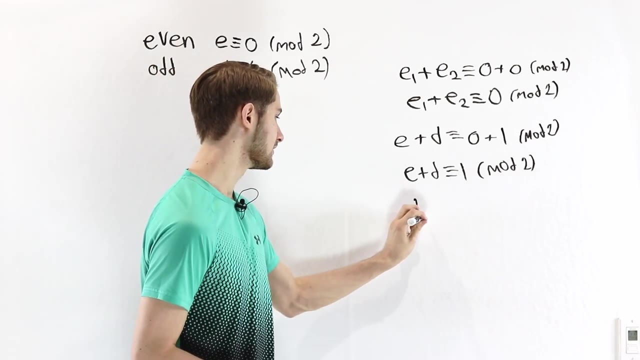 number plus an odd number is congruent to one mod two. We know if a number is congruent to one, then it is an odd number And therefore an even number plus an odd number will always be odd. Now we'll look at the last case, which is two different odd numbers. So say, we have D one plus D two. 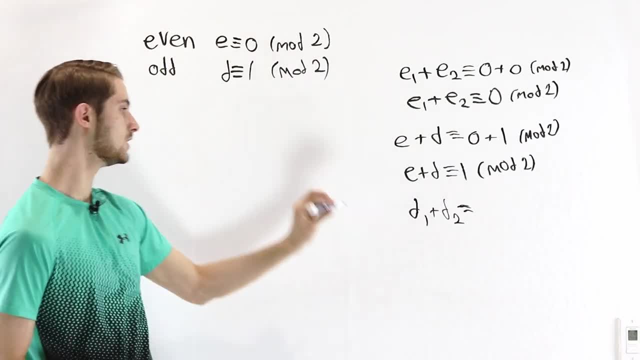 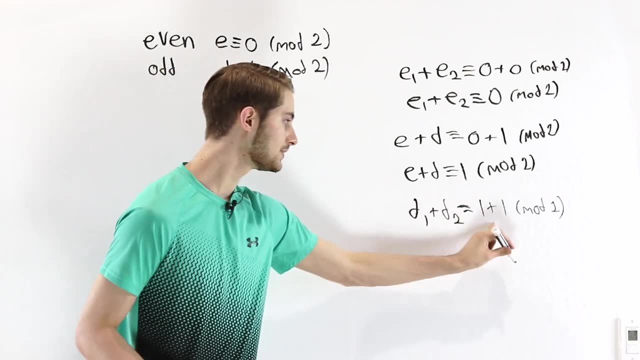 In that case, we know that both of these are going to be congruent to one mod two, So we have one plus one on the other side of our congruence, Of course, one plus one is equal to two, But because we're 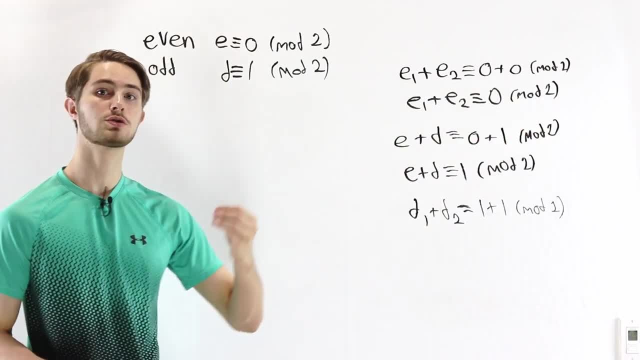 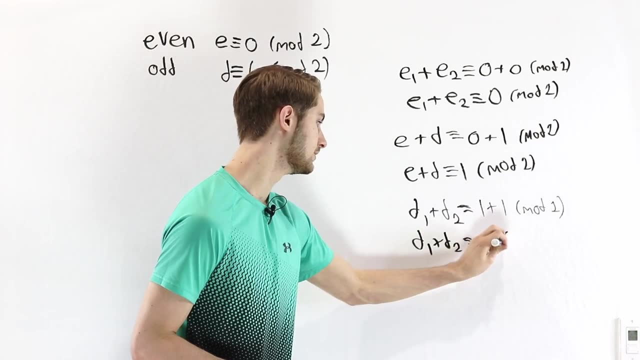 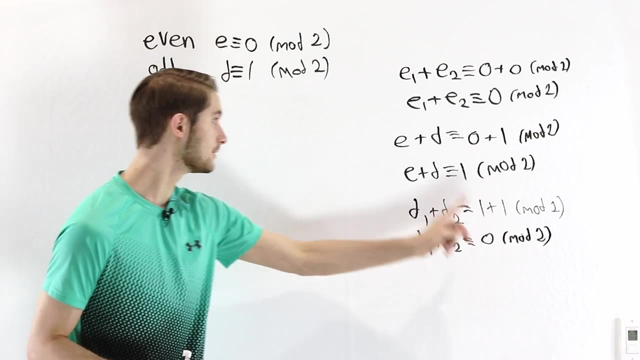 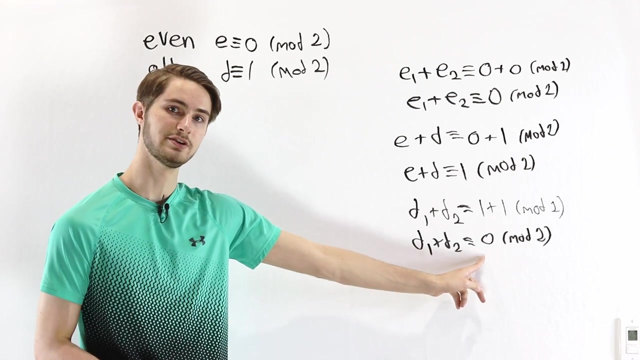 working with mod two, we know that two is congruent to zero mod two. So this sum of two odd numbers is congruent to zero mod two, because we know two is congruent to zero. And if this sum is congruent to zero, by definition it must be an even number And therefore the sum of two odd numbers is always. 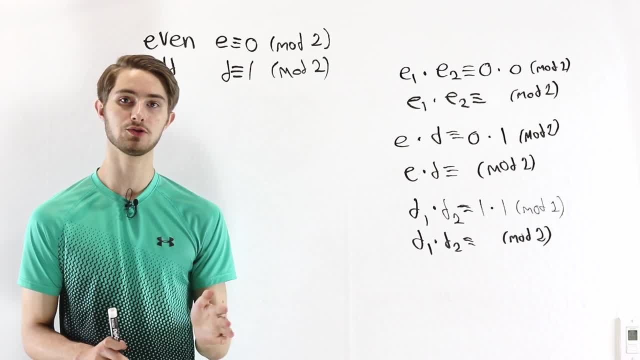 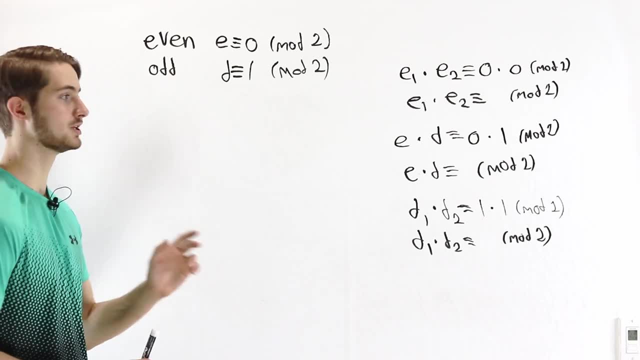 even So. now we're going to take a look at the rules for multiplying. What happens when we multiply two numbers that are either even or odd? We'll go through all the cases that we just saw. We know that an even number is congruent to zero and an odd number is congruent to one.